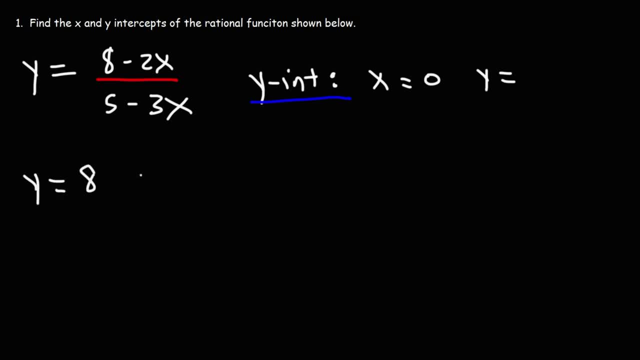 Let's go ahead and do that. So we're going to have 8 minus 2 times 0 over 5 minus 3 times 0. Now, 0 times anything is 0, so we simply get 8 over 5 as our answer. 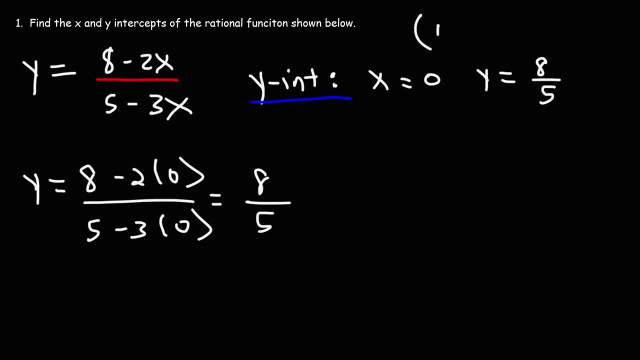 So that's the y-intercept. Now we can write the answer as an ordered pair. We can write it as 0 comma 8 over 5.. So that's all you need to do In order to find the y-intercept. 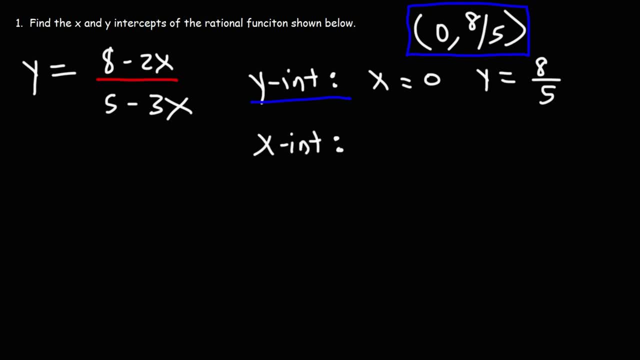 Now let's get the x-intercept. In order to find the x-intercept, set y equal to 0, and then solve for x. So we're going to have: 0 is equal to 8 minus 2x over 5 minus 3x. 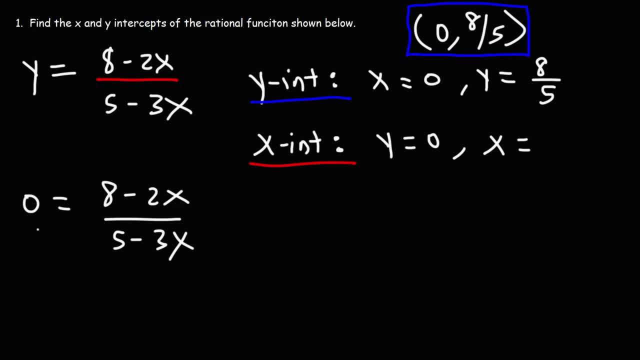 Now what I'm going to do is I'm going to rewrite 0 as a fraction. 0 is equivalent to 0 over 1.. Now we can cross multiply, So I have 1 times 8 minus 2x, which is just 8 minus 2x, and that equals 0 times 5 minus 3x. 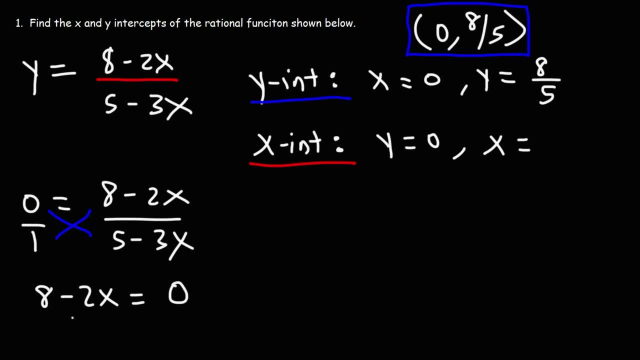 Now 0 times, anything is simply 0.. Next we can add 2x to both sides, So we get 8 is equal to 2x, And then to isolate x, we can divide both sides by 2.. So x is 8 over 2, which is 4.. 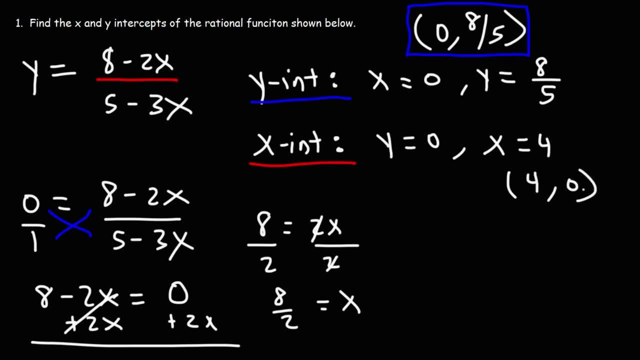 So the x-intercept is going to be 4 comma 0 as an ordered pair. So that's how we can find the x and the y-intercepts of a rational function. So remember, in order to find the x-intercept, set y equal to 0.. 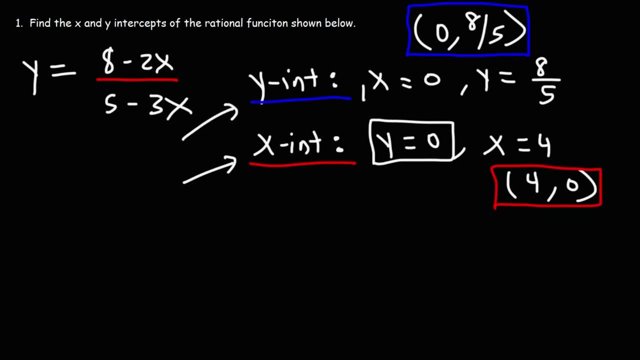 In order to find the y-intercept, set x equal to 0 and solve for y For the x-intercept after you set y equal to 0, then you can solve for x. Now let's try another problem. Let's say we have y is equal to 8 divided by x minus 3.. 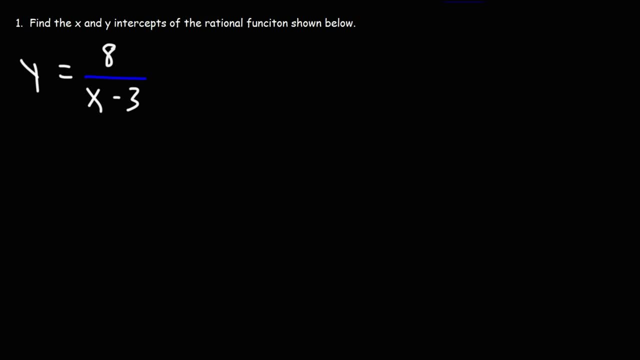 Go ahead and find the x and the y-intercepts for this particular rational function. So let's start with the y-intercept. So let's set x equal to 0. This is going to be 8 over 0 minus 3.. 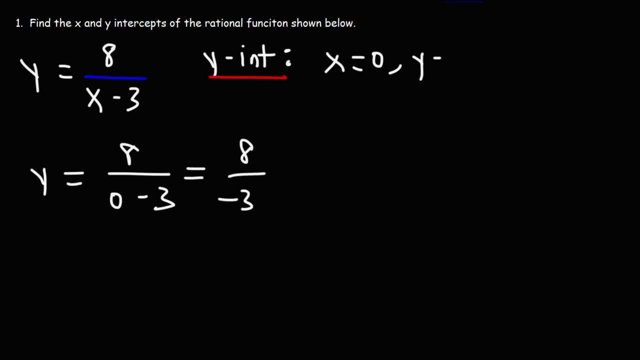 0 minus 3 is negative 3.. So we simply get negative 8 over 3.. So we can write our answer as 0 comma negative 8 over 3.. So that's the y-intercept for this particular problem. Now let's focus on the x-intercept. 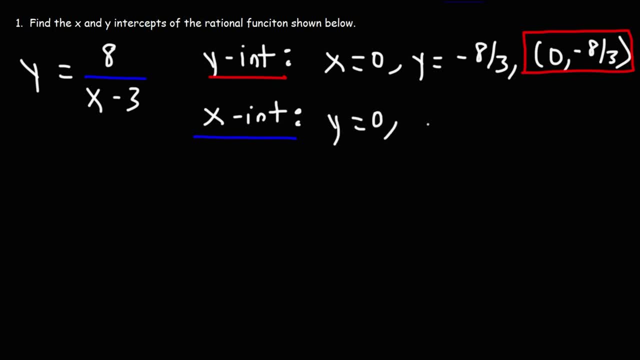 So this time we're going to set y equal to 0.. We're going to solve for x, So 0 is equal to 8 over x minus 3.. Let's put this over 1 and cross-multiply 1 times 8 is 8.. 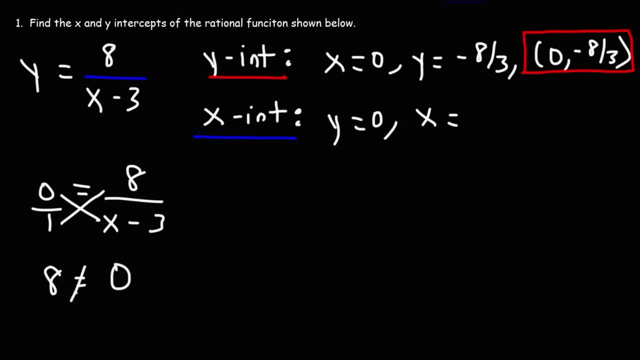 0 times x minus 3 is 0.. 8 does not equal 0.. So when you get an unequal expression like this, it means that there is no x-intercept. There's none. So that's it for this problem. 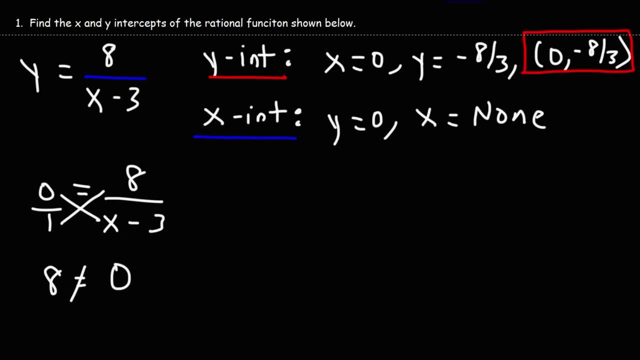 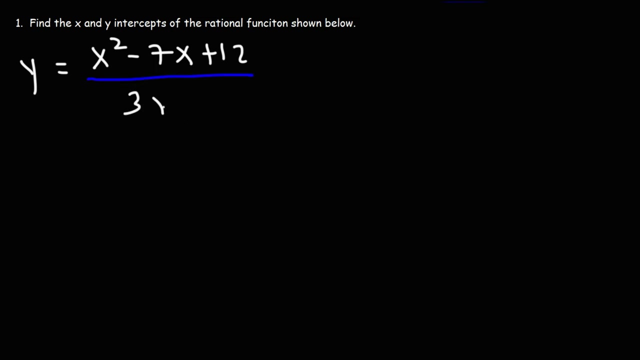 Now let's move on to the next one. Let's say we have: y is equal to x squared minus 7x plus 12.. And this is going to be divided by 3x squared minus 48.. So go ahead and find the x and y-intercept. 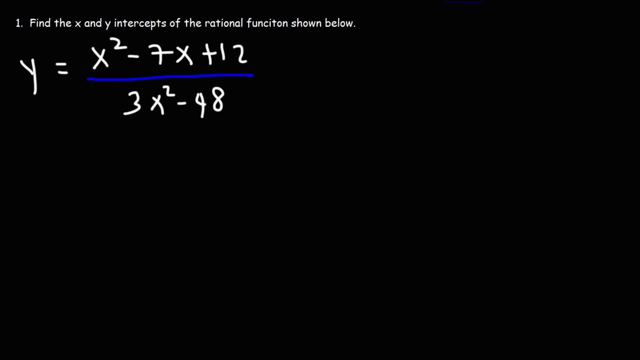 And we're going to use the y-intercepts for that particular rational function. Now, before we start this problem, we should attempt to factor every possible expression that we can, So let's go ahead and do that. It'll make the math a lot easier. 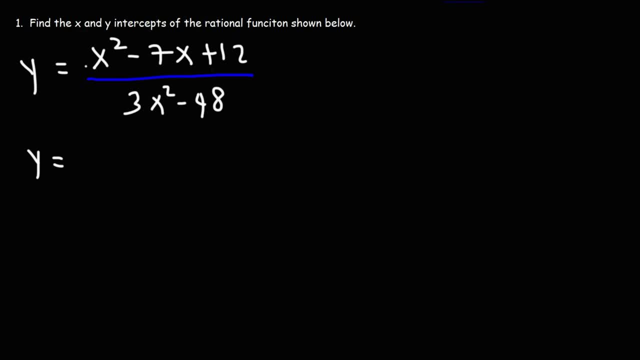 So how can we factor this trinomial where the leading coefficient is 1?? What we need to do is find two numbers that multiply to 12, but add to the middle coefficient Negative 7.. 4 times 3 is 12.. 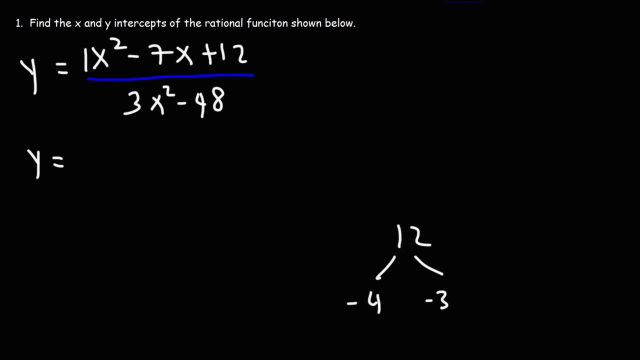 And the same is true for negative 4 and negative 3.. They multiply to positive 12. But they add to negative 7. So the factor of the numerator is going to be x minus 4 times x minus 3.. Now for the denominator. the first thing we need to do is take out the GCF. 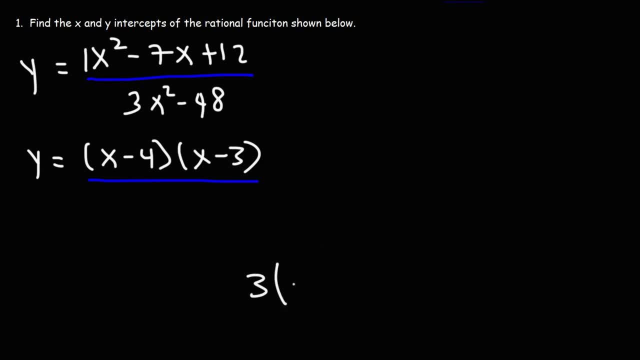 which is 3.. 3x squared divided by 3 is x squared Negative. 48 divided by 3 is negative 16.. Now we have a difference of two squares, So to factor it, it's going to be x plus 4 and x minus 4.. 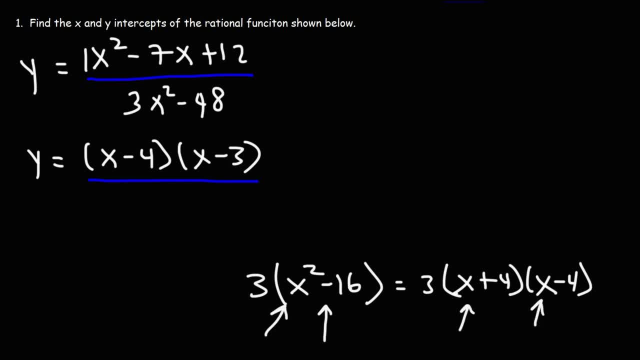 You take the square root of x squared, That'll give you x, And then the square root of 16 will give you 4.. One will be positive, The other will be negative. So notice that we have a common factor that we can cancel out. 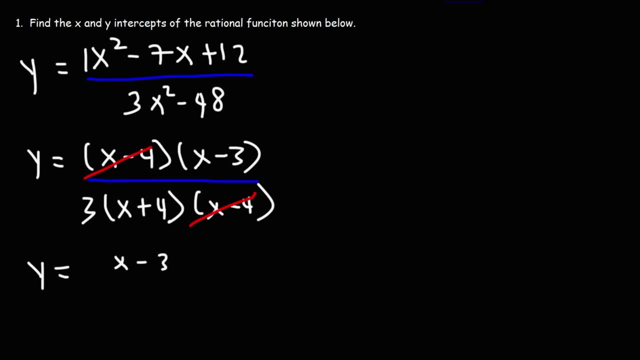 which is x minus 4.. So we're left with x minus 3 divided by 3x plus 4.. So now let's go ahead and find the y-intercept. So we're going to set x equal to 0, and we're going to solve for y. 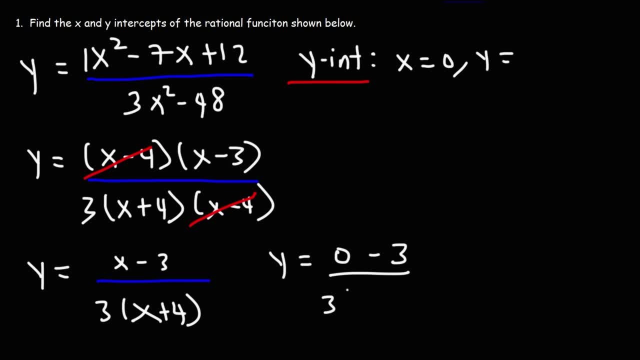 So this is 0 minus 3 over 3 times 0 plus 4.. 0 plus 4 is 4.. We could cancel a 3, and so we're left with negative 1 over 4.. So we can write the y-intercept as 0 comma, negative 1 over 4.. 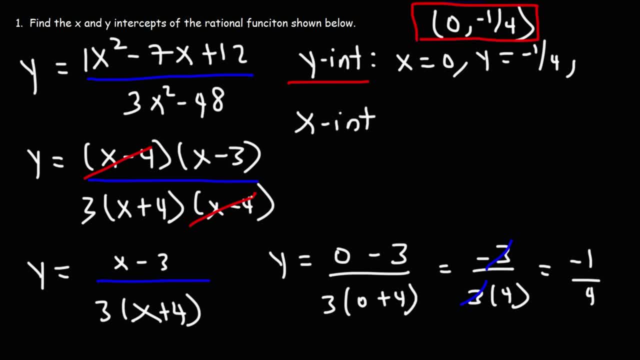 Now let's focus on the x-intercept. So this time we're going to set y equal to 0, and we're going to find x. So 0 is equal to x minus 3 over 3 times x plus 4.. 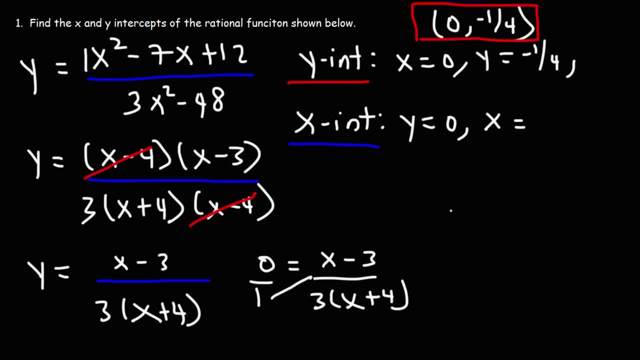 Just like before, we're going to put this over 1 and cross-multiply, So we have 1 times x minus 3, which is that, And that's equal to 0 times the stuff on the bottom, which will be 0..